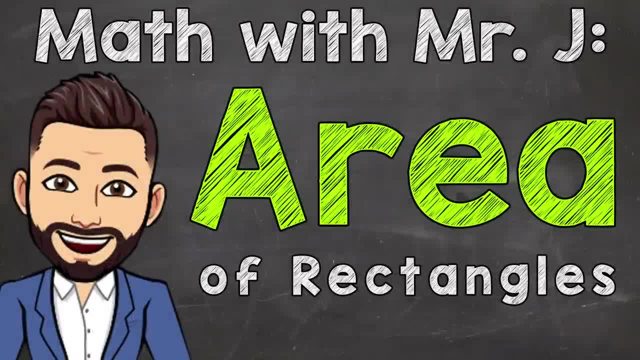 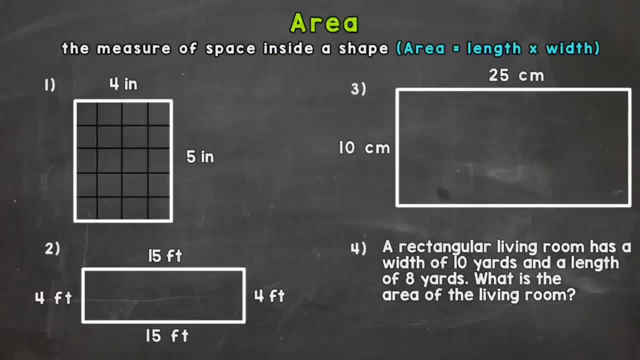 Welcome to Math with Mr J. In this video we're going to be discussing area and specifically how to find or calculate area of rectangles. And the area is the measure of space inside of a shape and that's up top for you to reference. there And in blue up top we have area equals length. 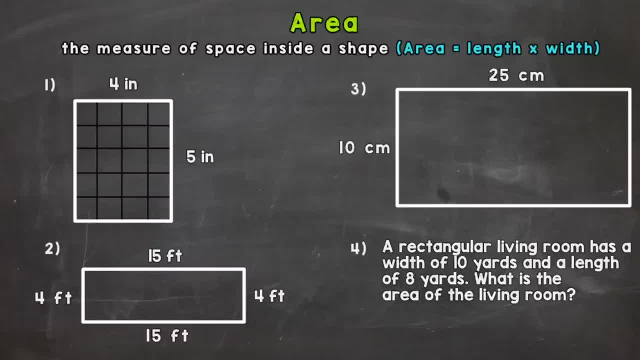 times width. That's the formula we're going to use to calculate area. So, as you can see, there are four problems on your screen that we're going to go through in order to learn more about finding area of rectangles. So let's jump right in to number one. So for number one, we have a. 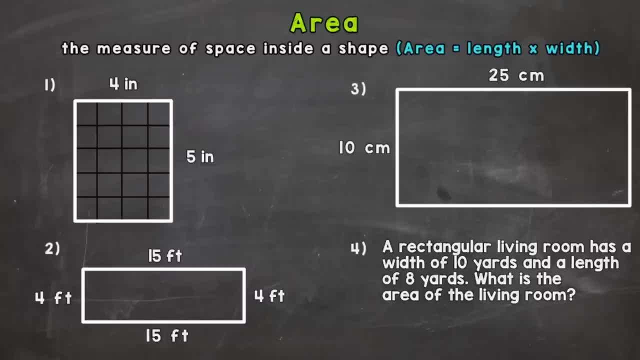 four by five inch rectangle. So the first thing we need to do in our calculating area problem here we write out our formula. So area equals length times width. Next we need to plug in our length and width. I'm going to use the four inches for the length and the five inches for the width. Now, if you flip, 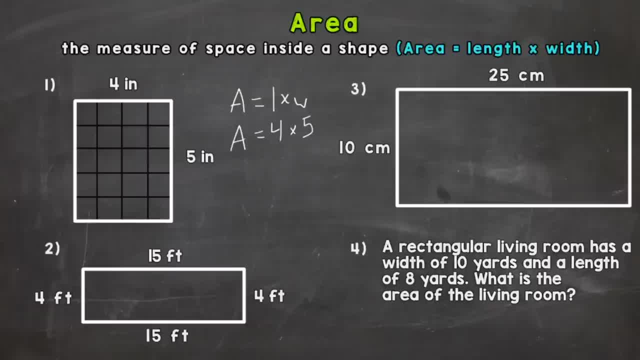 those and you use five for the length and four for the width. that's fine, You'll get the same answer either way. So after we plug in, we solve In order to calculate the area. So four times five gives us 20.. Now look back at the original problem. 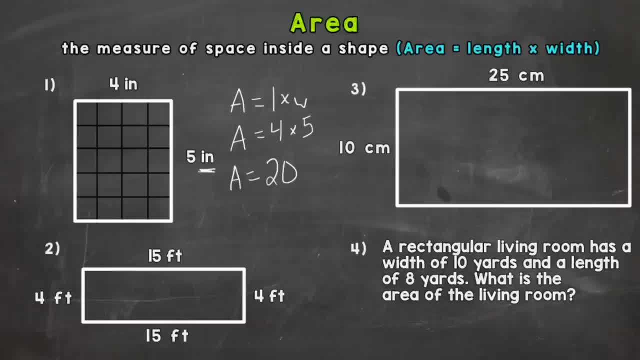 to see which unit of measure we used, And it was inches. So we have 20 inches and we put a little 2 up here for area And that tells us that the rectangle has an area of 20 square inches. And I did something so we can kinda visualize. 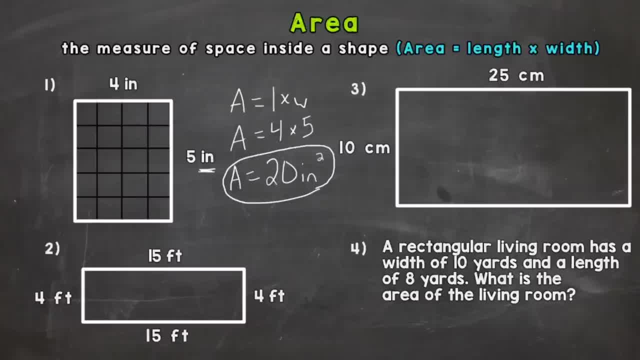 what those 20 square inches look like, that cover or fill that rectangle. So we have four inches going across, so I put four squares going across and we have five inches going down. So one, two, three, four, five. Now where all those lines intersect and create those squares, we have a 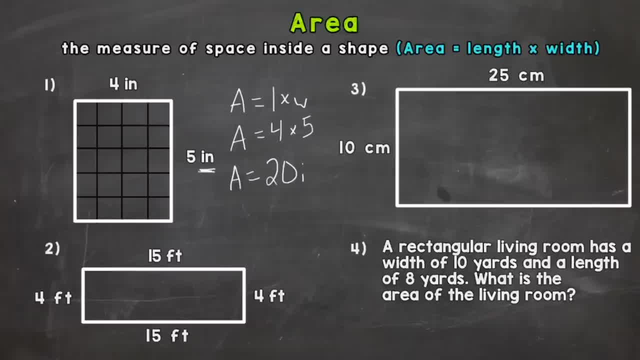 used and it was inches. So we have twenty inches and we put a little two up here for area and that tells us that the rectangle has an area of 20 square inches. And I did something so we can kind of visualize what those 20 square inches look like that cover or fill that rectangle. So we have four inches. 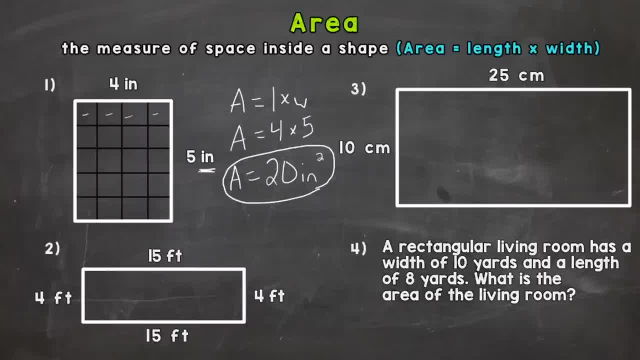 going across. so I put four squares going across and we have five inches going down. So one, two, three, four, five. Now where all those lines intersect and create those squares, we have a four by five rectangle and there are 20 squares that fill or cover that rectangle. Now it's much easier. 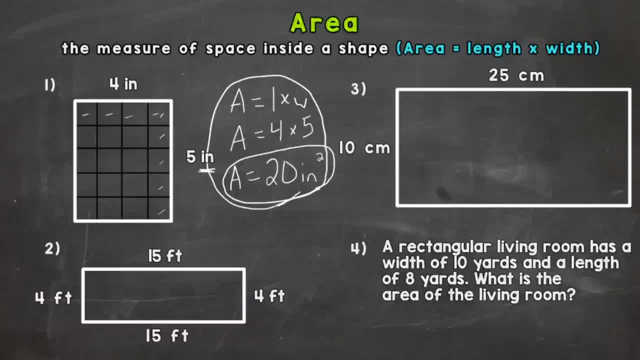 and quicker to just do four times five and follow our formula than fill a rectangle with all those squares. but this kind of shows us what those 20 square inches look like that fill that rectangle. Let's take a look at number two. So we write out our formula first. 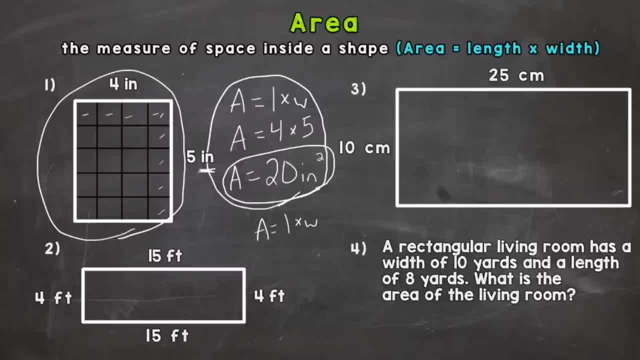 area equals length times width. Next we plug in. Now this is a little different than number one, because we have all sides the measurements listed. Do not just multiply everything for an area problem. You have to pick out the correct length and width. If you just multiply everything, 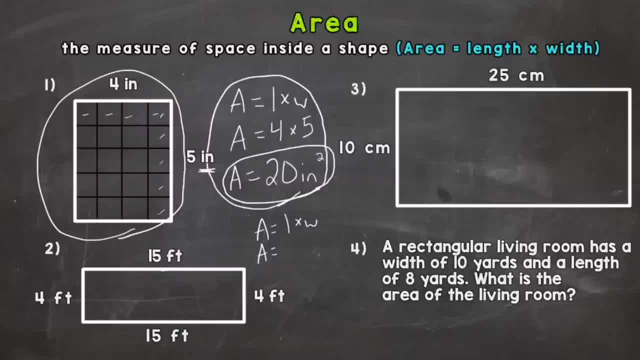 you're not going to get the correct answer. I'm going to use 15 feet for the length times four feet For the width. 15 times four equals 60 square feet, and that's going to be our answer for the area to number two. So let's take a look at number three. Write out our formula first. 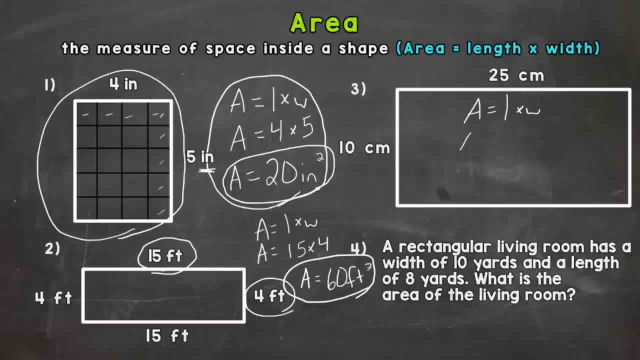 area equals length times width. Plug in. I'm going to use 25 for the length times length, 10 for the width. Solve to find our area: 25 times 10 equals 250, and that is square centimeters. So area equals 250 square centimeters. So for number four, we have a word problem where 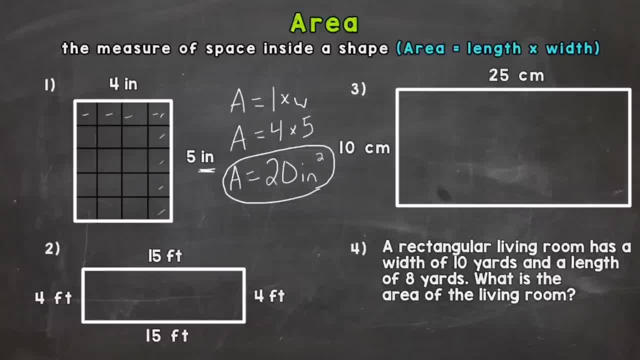 four by five rectangle and there are 20 squares that fill or cover that rectangle. Now it's much easier and quicker to just do four times five and follow our formula than fill a rectangle with all those squares. but this kind of shows us what those 20 square 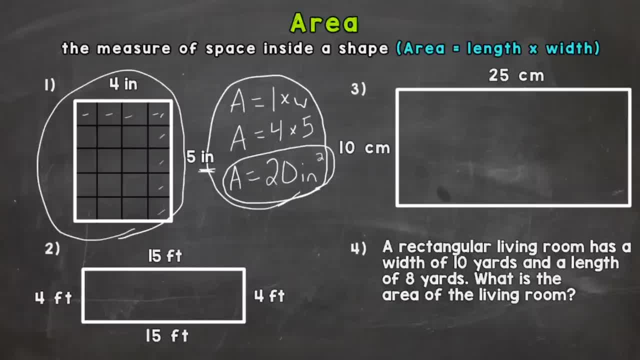 inches look like that. fill that rectangle. Let's take a look at number two. So we write out our formula: area equals length times width. Next we plug in: Now this is a little different than number one because we have all sides the measurements listed, Do not? 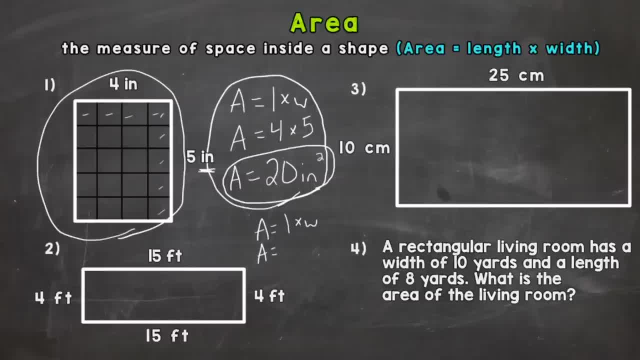 just multiply everything for an area problem. You have to pick out the correct length and width. If you just multiply everything, you're not going to get the correct answer. I'm going to use 15 feet for the length times 4 feet for the 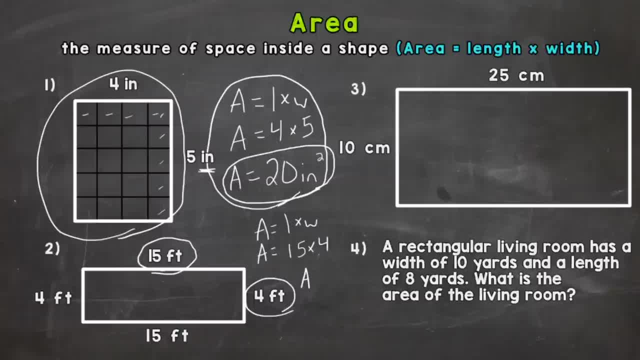 width 15 times 4 equals 60 square feet, and that's going to be our answer for the area to number 2.. So let's take a look at number 3.. Write out our formula. first: Area equals length times width. 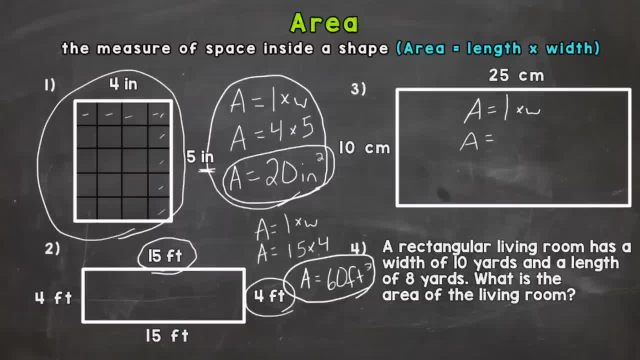 Plug in. I'm going to use 25 for the length times 10 for the width. Solve to find our area: 25 times 10 equals 250 and that is squared centimeters. so area equals 250 square centimeters. So for number 4 we have a word problem. 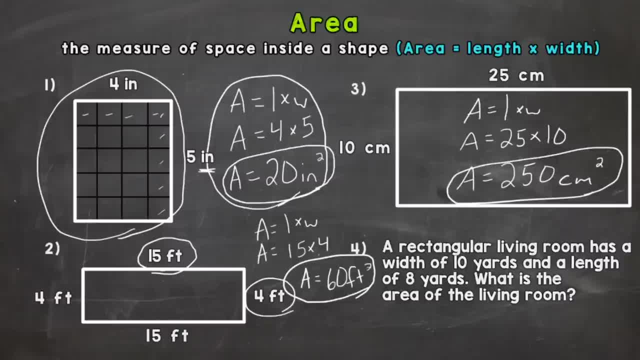 where we're going to need to calculate the value of the area. So we're going to need to calculate the value of the area. So area equals 250 square centimeters. For number 4 we have a word problem: area. so a rectangular living room has a width of 10 yards and a length of 8. 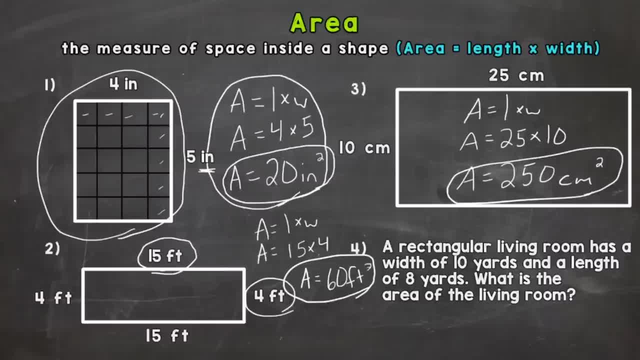 yards, what is the area of the living room? so first step, we need to write out the formula: area equals length times width. then we need to plug in: length of 8 yards times width of 10 and then solve: so, 8 times 10, the area equals 80 and